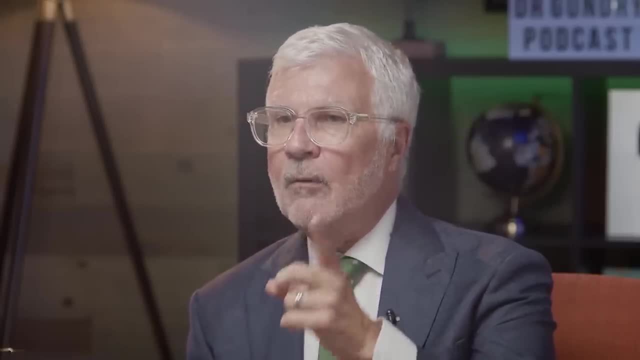 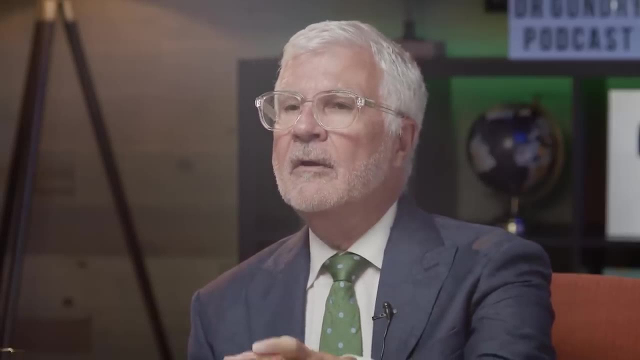 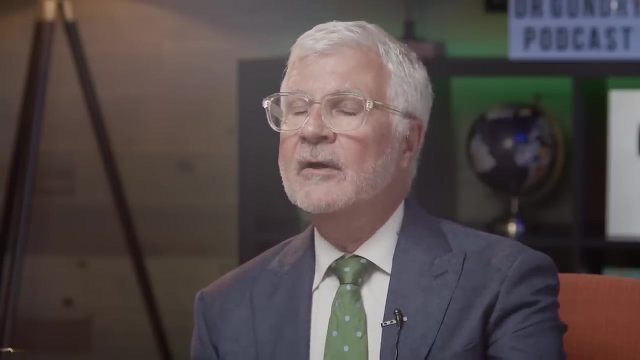 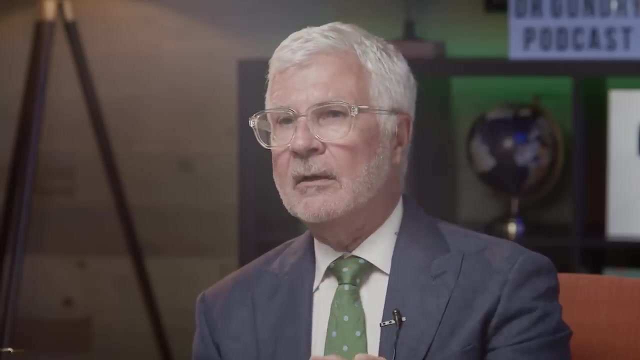 it into a baboon Because of that one dumb sugar molecule. if I take a pig heart and put it in a baboon, that pig heart will stop in about five hours from acute rejection because the baboon's white blood cells attacked that, that sugar molecule in that pig heart. 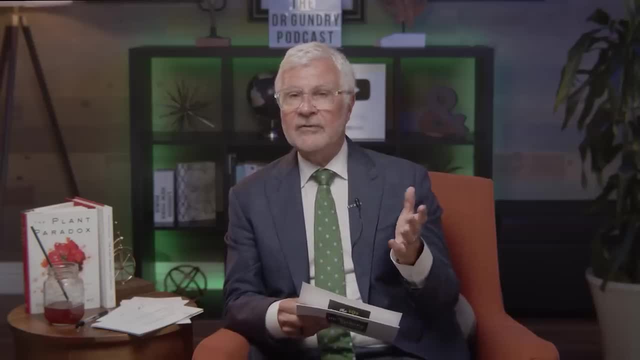 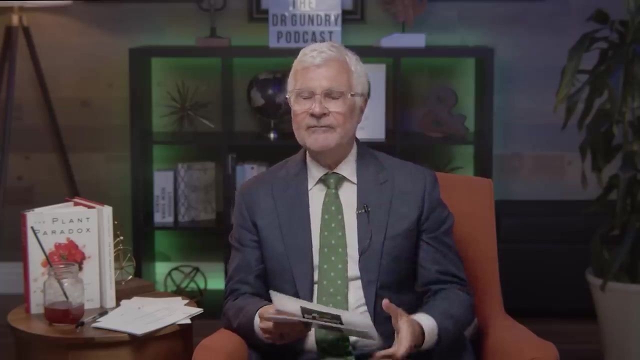 Now, you may remember, I'm pretty famous for getting around that system. I've had untreated pig hearts live for a month in baboons using my tricks, But that sugar molecule promotes an antigenic response. So whenever we eat new 5G-containing foods, 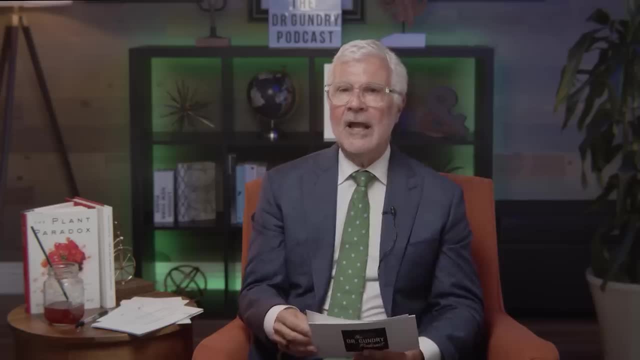 like a steak, like bacon, like lamb. we actually make an antibody to our own blood vessels And there is interesting reasoning that part of the reason that meat eaters have more coronary artery disease than non-meat eaters is because of new 5Gc in an autoantibody response. 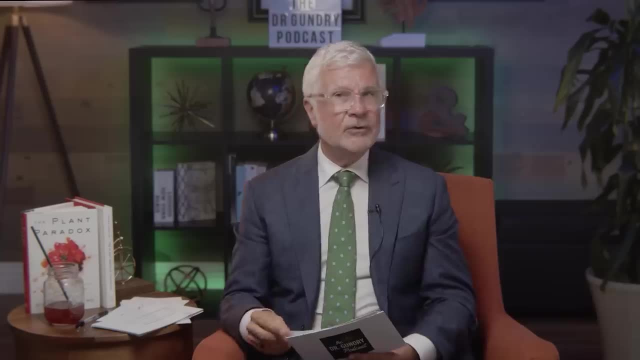 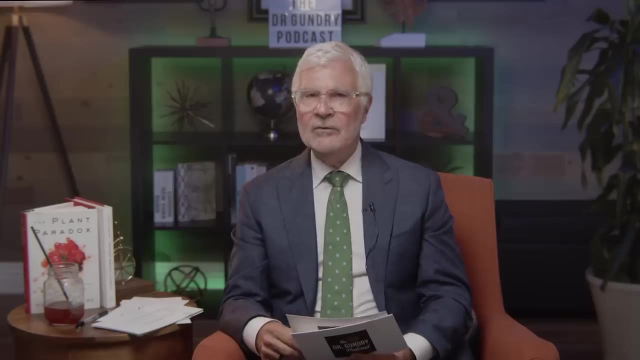 against our own blood vessels. That's number one. Number two: tumors are known to use new 5Gc to cloak themselves so that they won't be seen by the immune system. Now you already know. we don't manufacture new 5Gc. 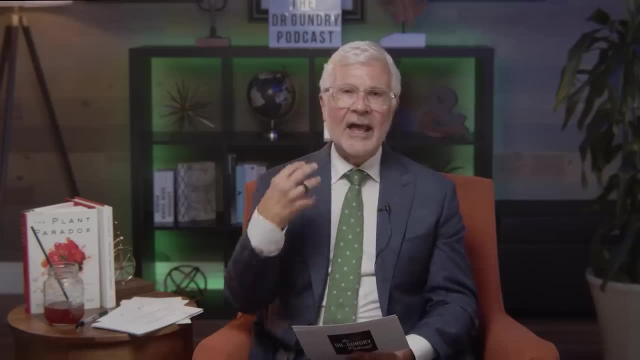 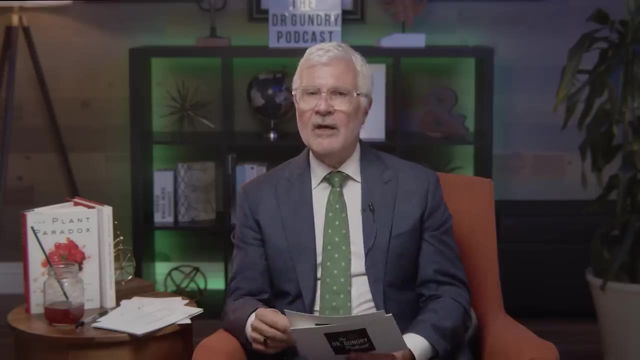 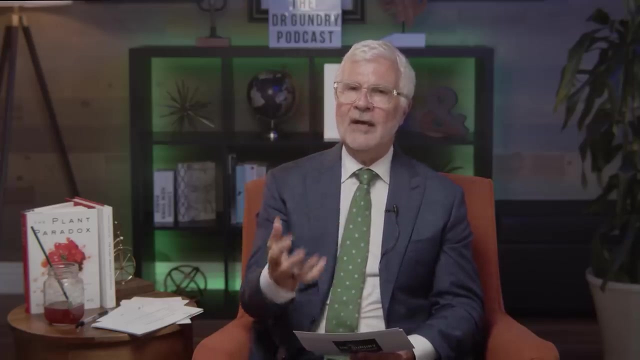 which means that tumors in us had to acquire new 5Gc from the foods we eat, And that's why there are- there are a number of studies that show a correlation between red meat eating and increased cancer risk. Now you've heard me say over and over again: 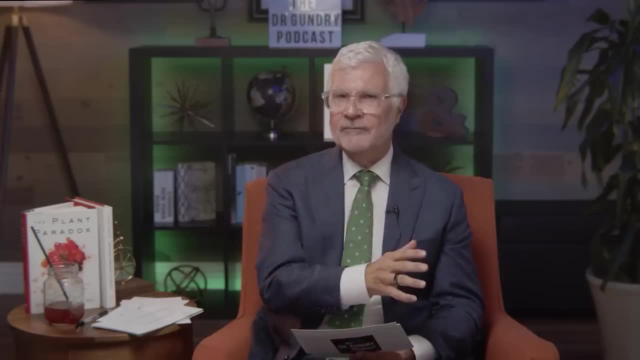 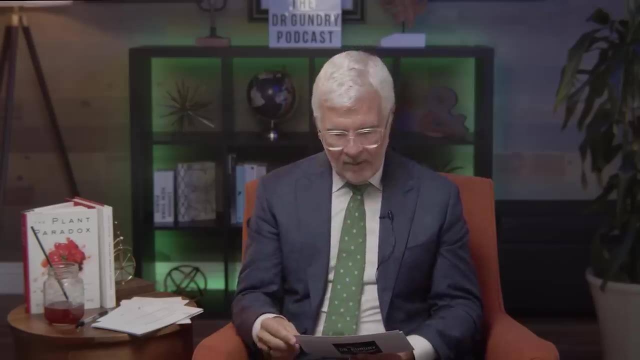 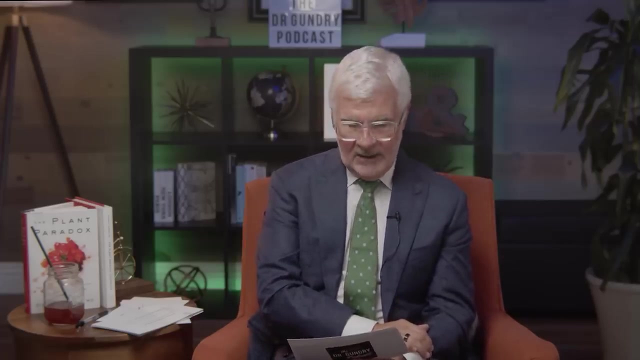 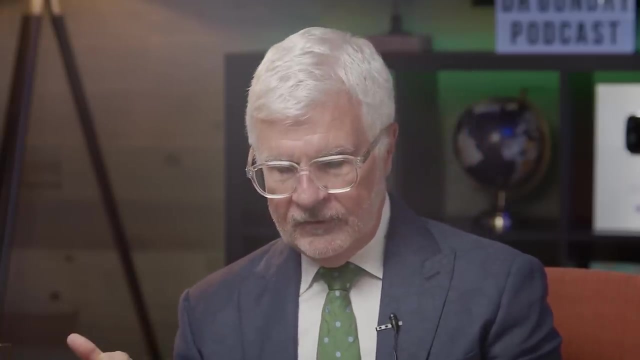 correlation does not mean causation, But there's enough of a reasoning behind this that it's probably not your friend. Now, if you are going to eat meat- yes, even I eat meat- Then abide by the following principles: First of all, shellfish and fish and chicken. 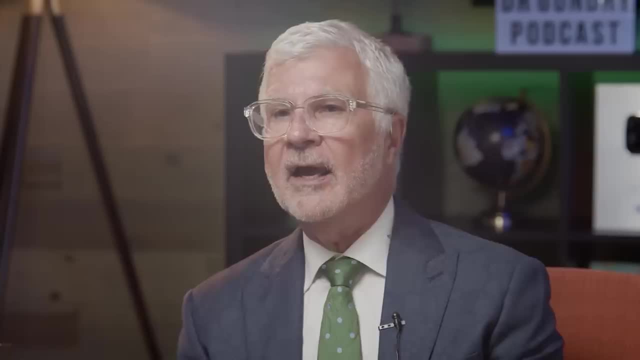 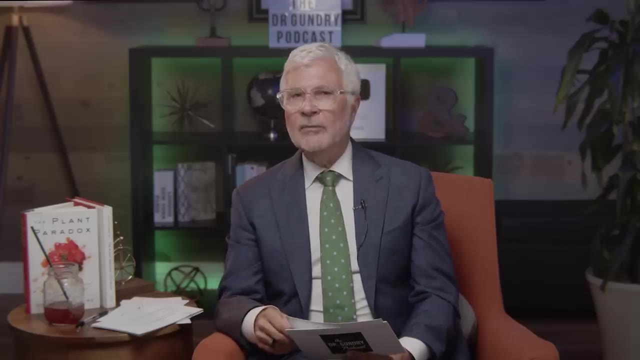 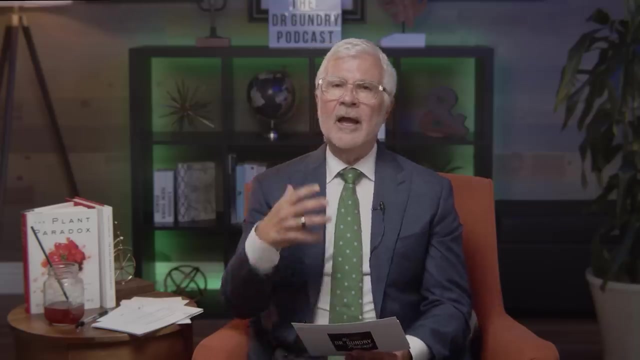 do not have new 5Gc. They have new 5AC, just like us. But also keep in mind that animal protein, regardless of the animal, regardless of whether it was a fish or a chicken or beef, has a large amount of protein. 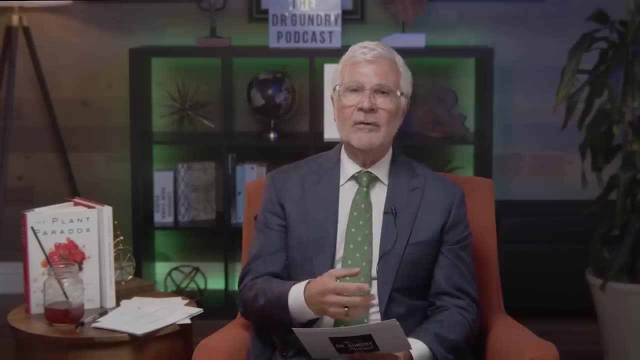 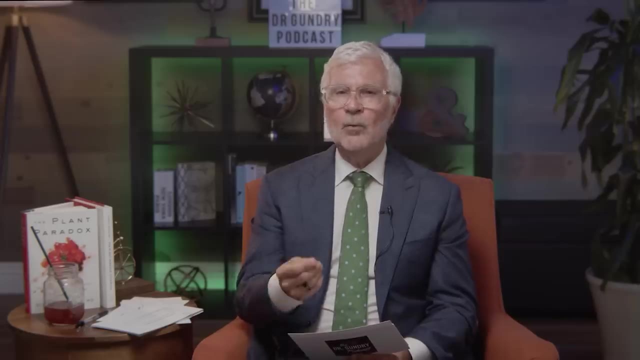 It's a large amount of a protein and amino acid called methionine, And there is strong evidence that methionine is one of the drivers of aging And it stimulates a receptor in us called mTOR, the mammalian target of rapamycin. 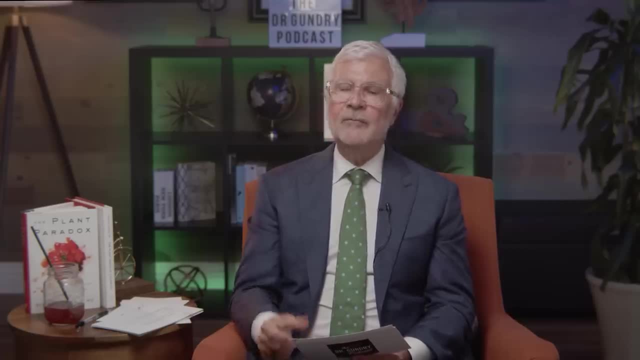 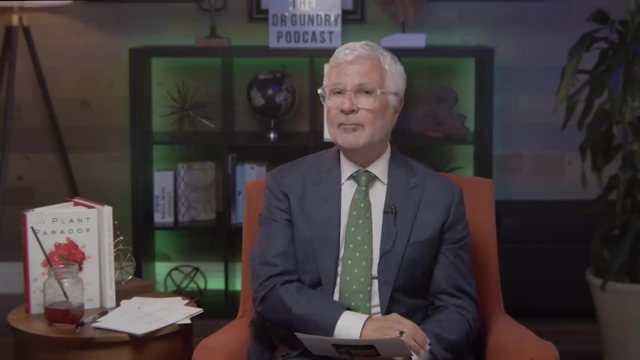 And there again is strong evidence that removing methionine from, say, a pig's diet will allow that pig to live 50% longer than a pig who eats a methionine-enriched diet. 50% longer by removing methionine. 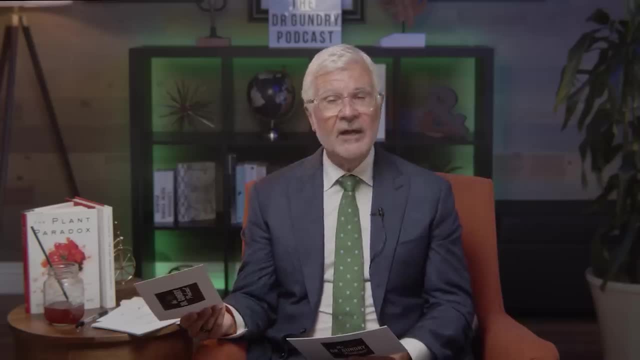 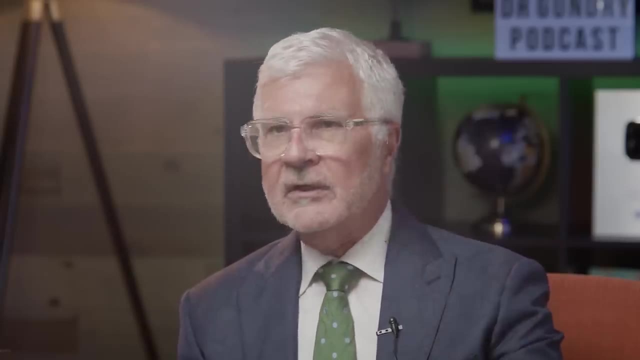 And plant proteins have far less methionine than animal proteins. Okay, I don't care, I still want my piece of chicken, I want my piece of fish, I want my beef, I want my fish, As, like I always say, 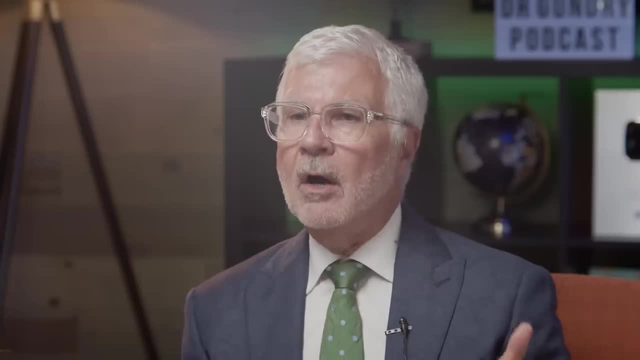 you are what you eat, but you are what the thing you're eating ate. Now that means that a cow that was fed a diet of grains and corn, even if it was organic grains and corn, will be a giant lectin bomb, will be a giant inflammatory fat bomb. 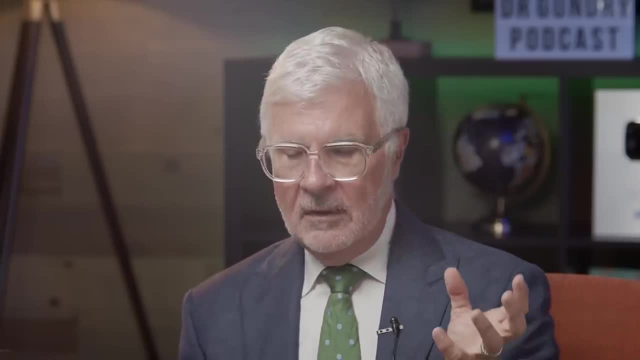 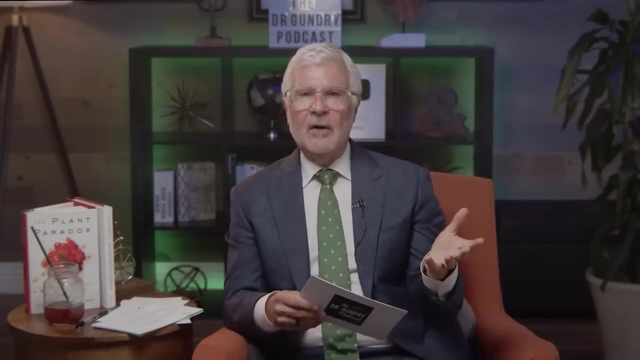 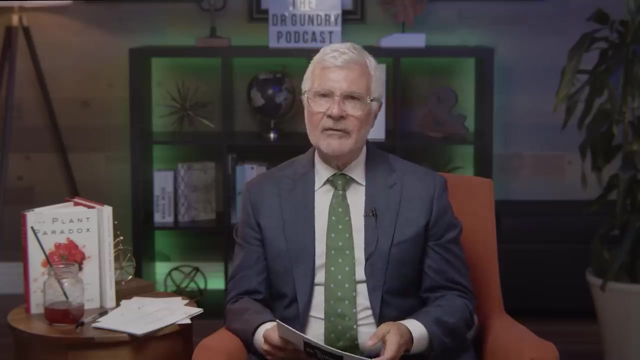 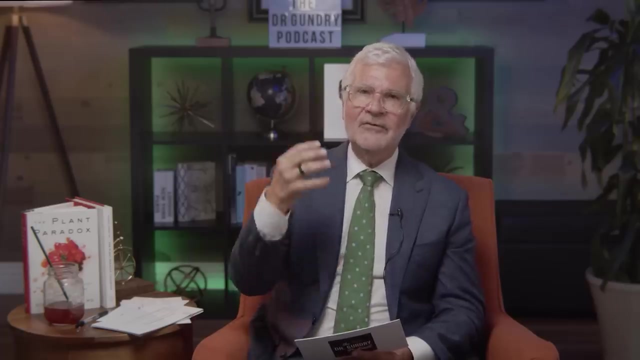 because the corn and grain is now part of that meat. Similarly, if you get a farm-raised salmon or an organic farm-raised salmon, it is fed organic corn and soybeans And rather than omega-3 fats that a salmon would give you from the wild, that salmon. 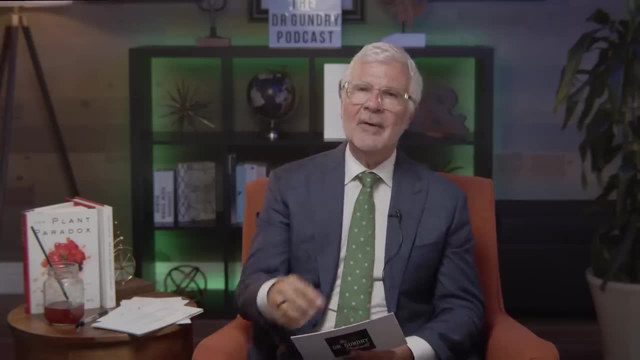 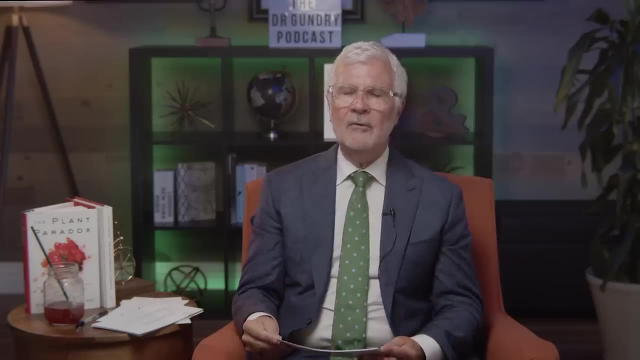 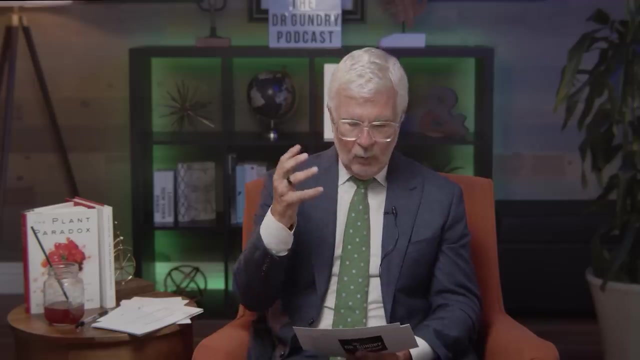 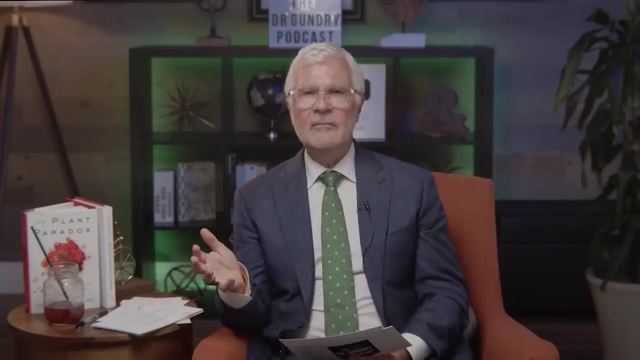 will actually give you inflammatory omega-6 fats because you've fed it omega-6 fats in the corn grain and soybeans. So just the word organic doesn't cut it. You got to have wild. Similarly with chicken. just because it says organic free-range means absolutely nothing. You have to. 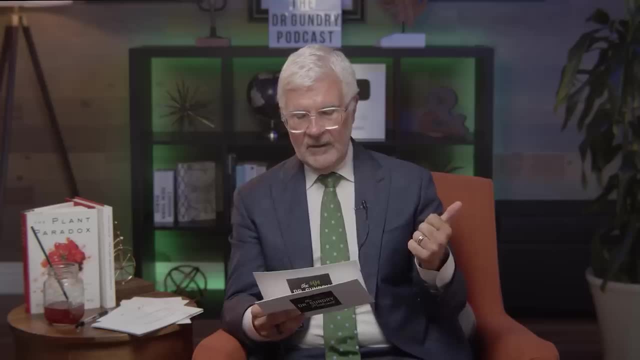 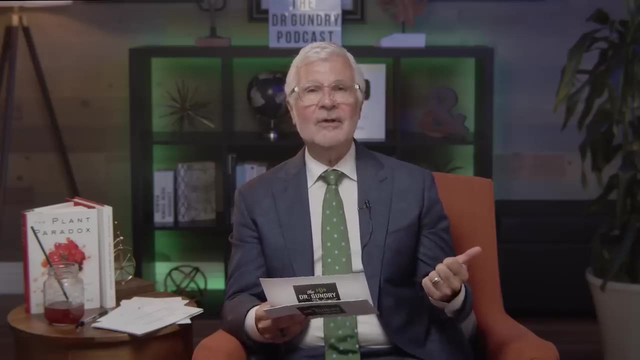 look for pasture-raised poultry And, quite frankly, there are now lectin-light chickens. You can go to lectin-light chickens. You can go to lectin-light chickens. You can go to lectin-light chickens- lectin-lightchickenscom Farmer Dan, we've had him on the podcast and get chickens that are not fed. lectin-containing foods. Northstar also sells a soy corn-free turkey. If you decided that you want new 5GC in your diet, then please look for grass-fed, grass-finished beef or bison or lamb. Now, it's very difficult to find true pastured grass-fed pork. It can be done. There are porks. 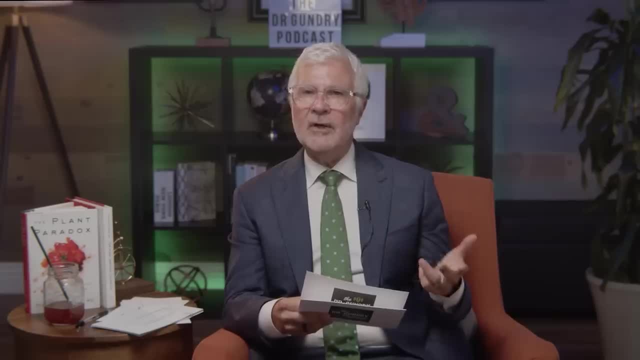 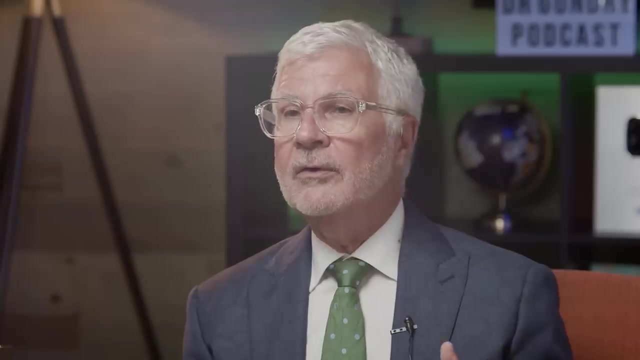 that are remarkably safe, particularly Iberico pork from Spain, sometimes called 5J. This is prosciutto that has been fed acorns, And if you're actually in Spain or Portugal, you can actually buy hams and pork products that have been strictly fed acorns, which have an amazing omega-3 profile. 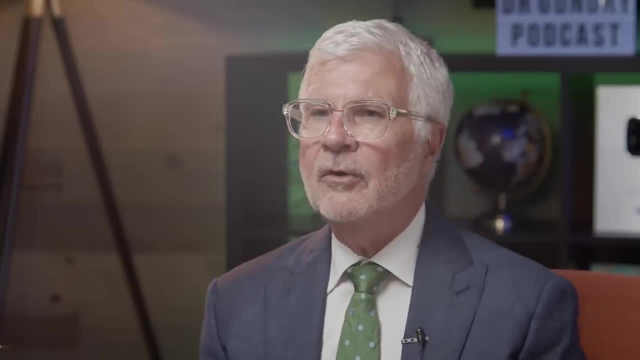 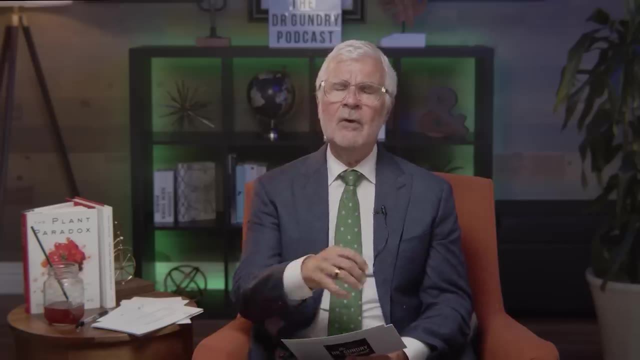 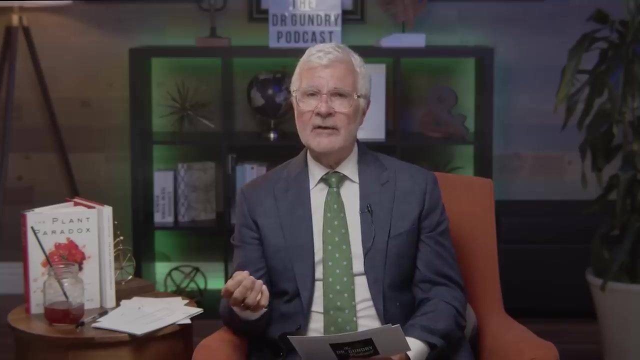 Now, similarly, prosciutto hams, prosciutto pigs, are fed the rinds of Parmesan cheese as part of their diet. So prosciutto di Parma is actually pretty doggone good for you, And it's regulated Now just. 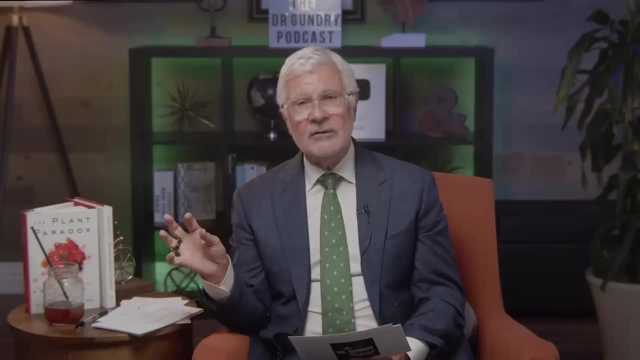 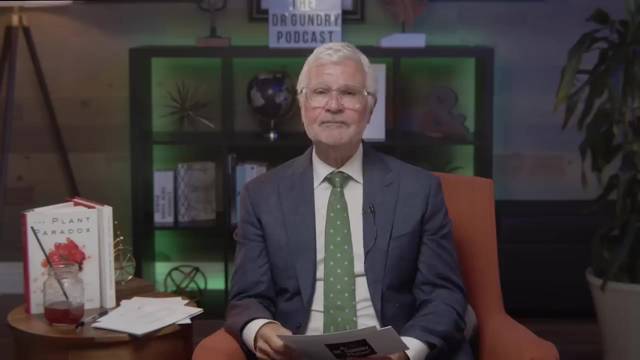 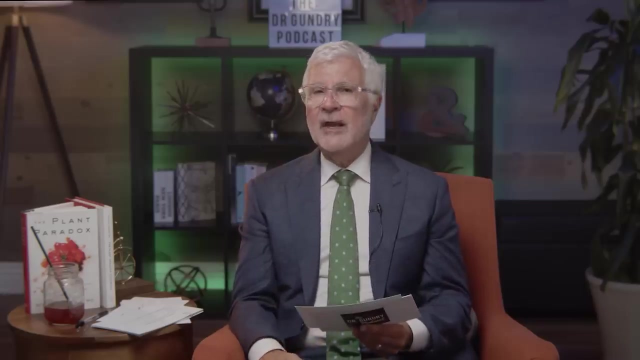 because something is labeled prosciutto. you gotta look at the label and find out where it came from. American prosciutto is not raised the same way as prosciutto di Parma, So look for that on the label. Most lamb from New Zealand is grass-fed. About 80% of lamb from Australia is grass-fed. Goats and sheep in. general, do not like eating grains. Goats love weeds, So goat products are actually one of your best choices. Are there other healthy meat alternatives? Yeah, Upton's natural jackfruit Corn, which is mycelia mushroom-based. Get the corn that doesn't have any breading. My favorite, quite honestly, is grounds. It tastes like ground. turkey. It works like ground turkey. It tastes like ground turkey. It works like ground turkey. It works like ground turkey. It works like ground turkey. It makes your tacos your lettuce tacos. please out of it. Hilary's root burger is great. Now, please, please, please, avoid fake meats like Beyond Beef and the Impossible Burger. These have glyphosate, they have soy, they have genetically engineered heme, And the last thing you want is a processed-plant food That's to look like a burger. It may be from plants, but it is processed nonetheless.